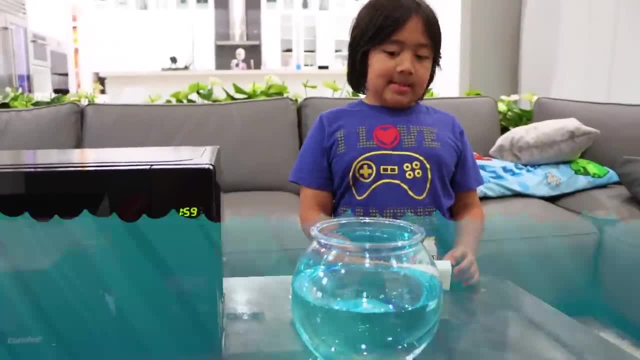 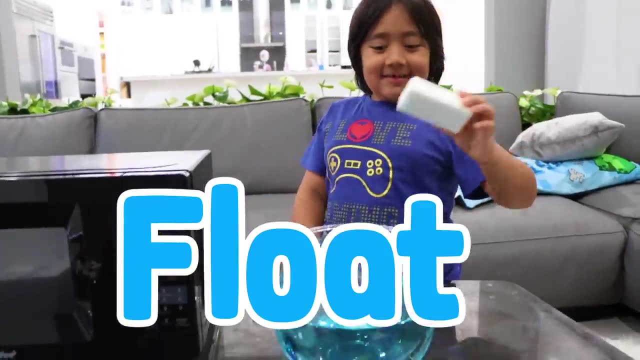 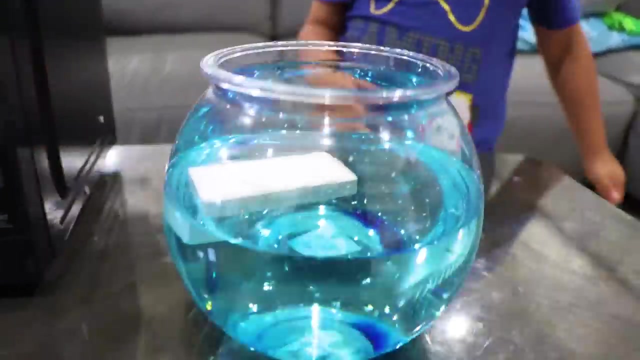 ivory soap into water And first we're going to see if it's going to sink or float, Okay. Okay, Do you think it's going to sink or float? Maybe float? Okay, Let's try it. It's floating. Yes, there it is. It actually floats in water. 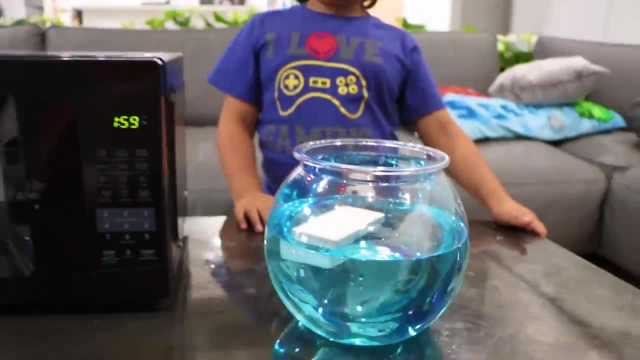 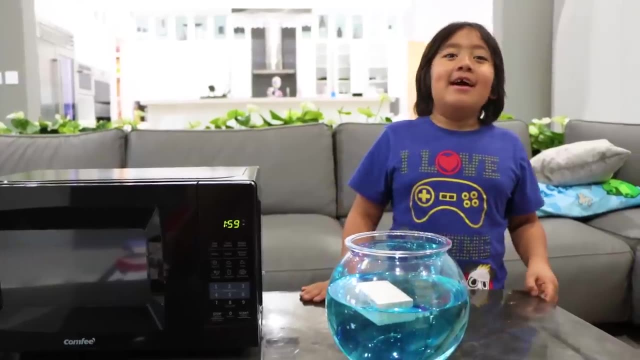 We don't have other other bars of soap, but if you have a different brand you can see if it also sinks or floats. These are ivory brand. So what does it mean when it floats on water More dense or less dense than water? 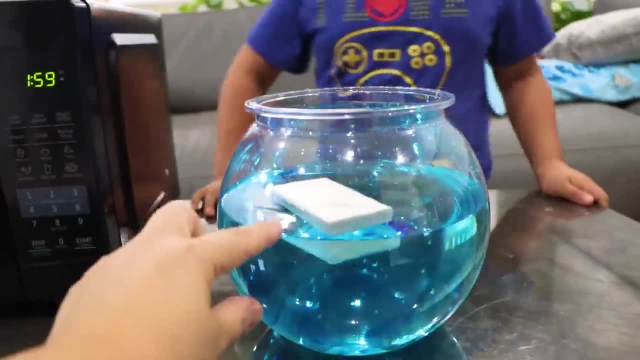 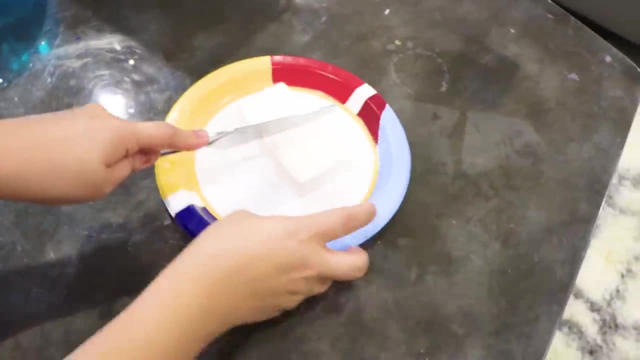 Less dense. Good job, The bar of ivory soap floated because it's less dense than water, probably because there's lots of air holes inside. okay, So we're actually gonna cut it open and see. Okay, I'm gonna cut the bar of soap in half. 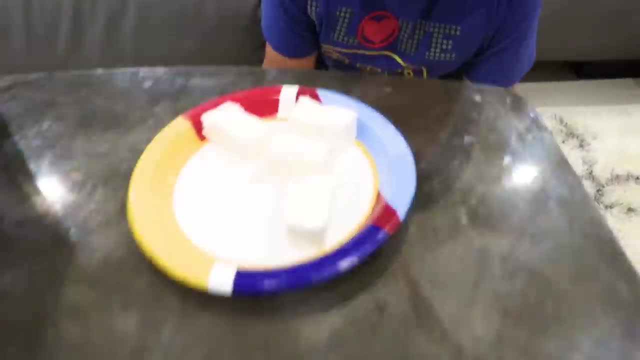 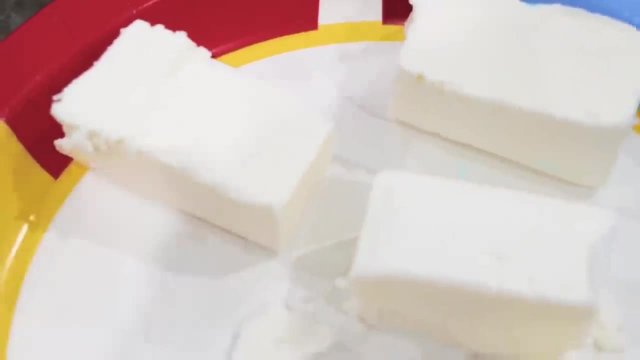 Okay, all right, so I cut it more. If you examine it very closely, it has like little holes of emptiness. I guess it's where all the air is. Are you ready to microwave it? Yeah, All right, we got our new ivory bar of soap here. 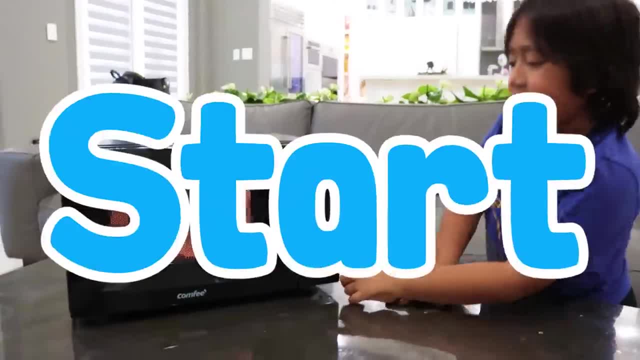 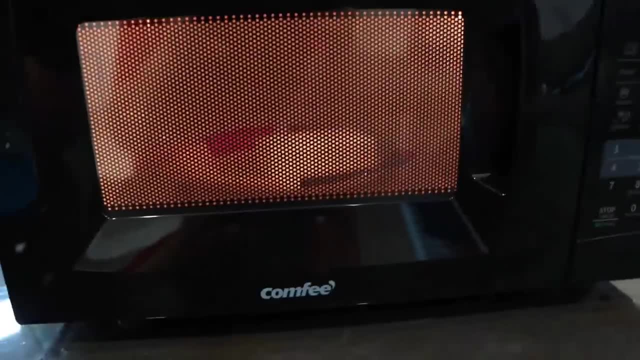 Put it in the microwave, closing it, Start. There we go. all right, We are keeping our eyes on the bar of soap. Make sure you use a microwavable safe plate. Okay, let's see. See, There's like stuff coming out of it. 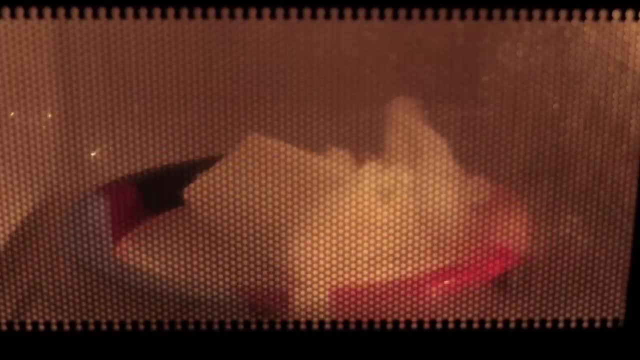 It's hard to see because of Do you see, like the stuff? Oh, I do see. You guys see Whoa, keep your eyes on it. Look guys, it's a little bit hard to see, but look, it's expanding. 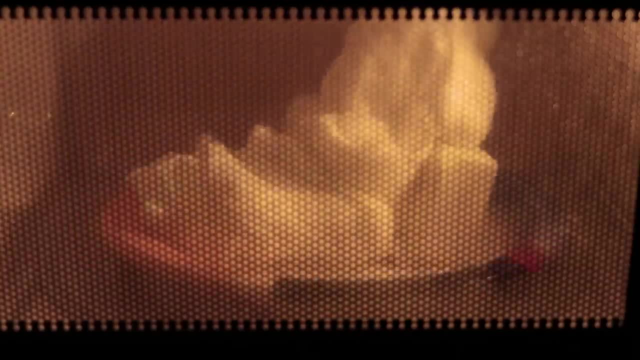 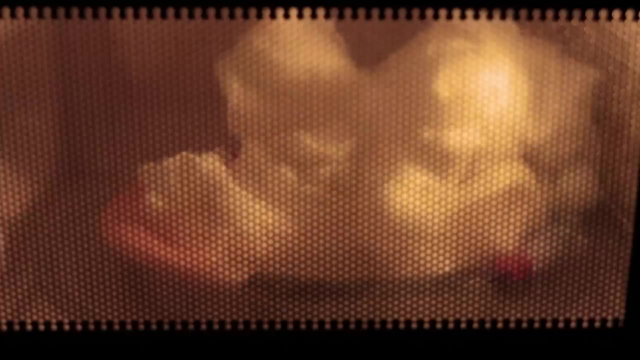 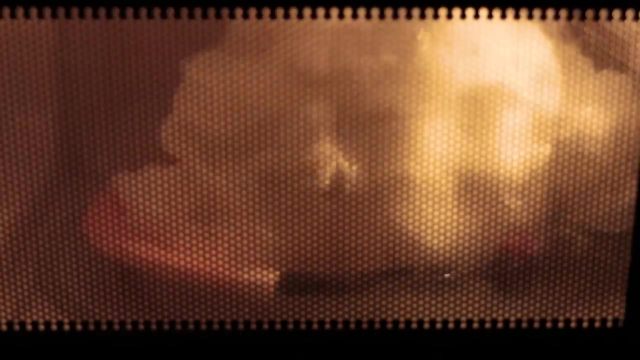 Yeah, it's expanding by a lot. Whoa, I think it's melting the soap or something. Whoa guys, look That's big. Should we stop it? It's gonna go all over the microwave. Stop, Whoa guys, look at this. 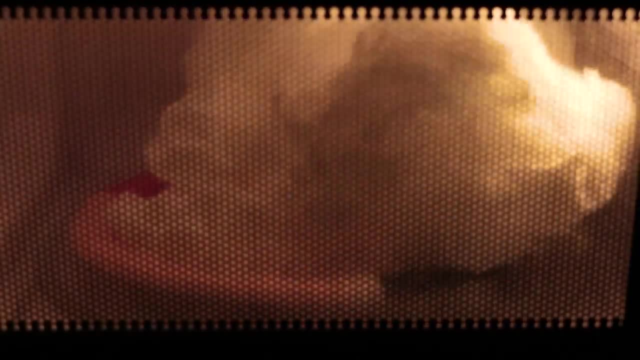 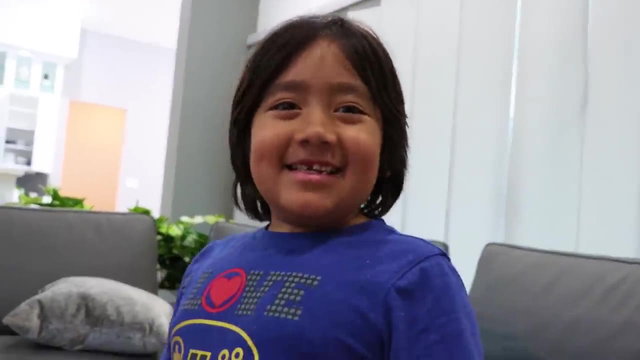 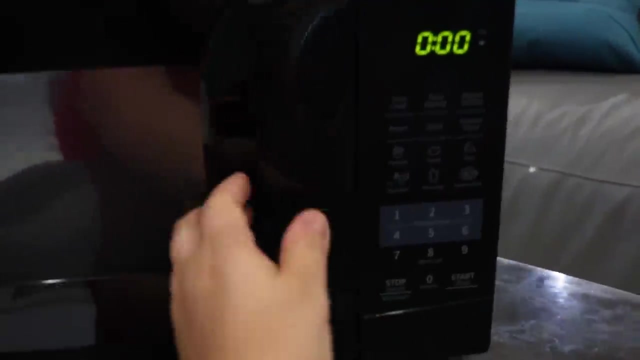 Whoa, whoa, it's like it's the whole microwave. Oh, Do you smell anything? A little bit Smells like soap. Yeah, Whoa, it looks fluffy like marshmallows. Okay, done, Okay, Okay. only adults do this, because it might be hot. 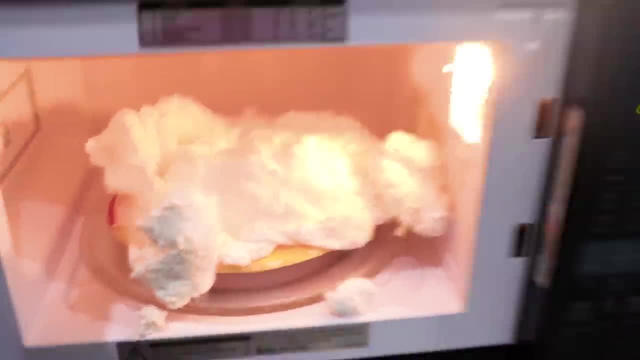 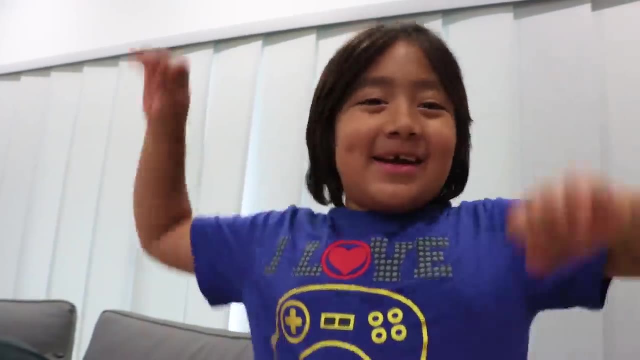 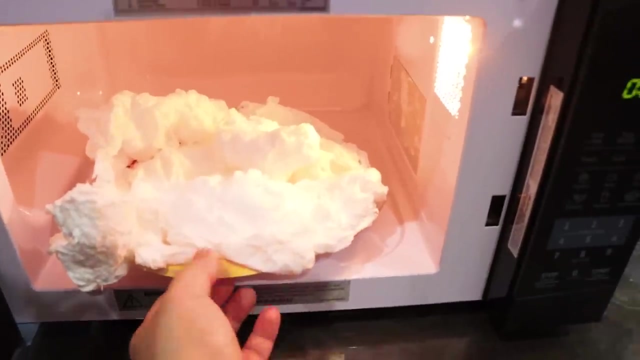 Oh, Whoa, Whoa, Whoa. Did you expect that? No, So what happened? It got melted and then it got bigger. It expanded, Yeah, Yeah, Look, super expanded. Look at that. Okay, only adults touch this. 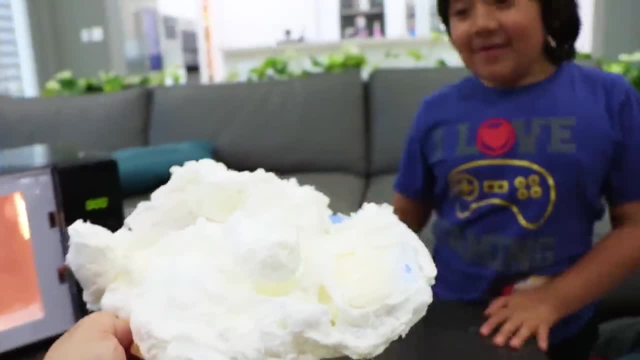 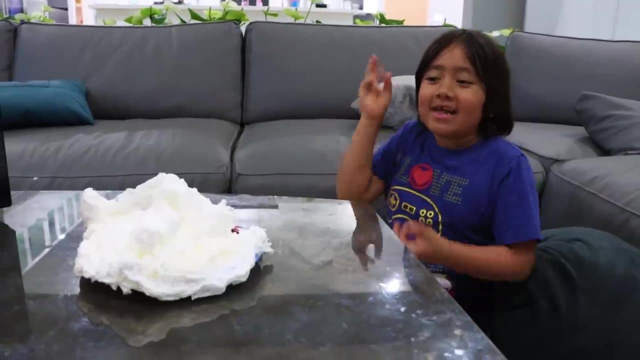 It might be hot. Whoa, don't touch it yet. okay, It might be hot. Okay, we're gonna wait for a little bit. but just looking at it, what does it look? like Toilet paper that you like? scramble it a lot. 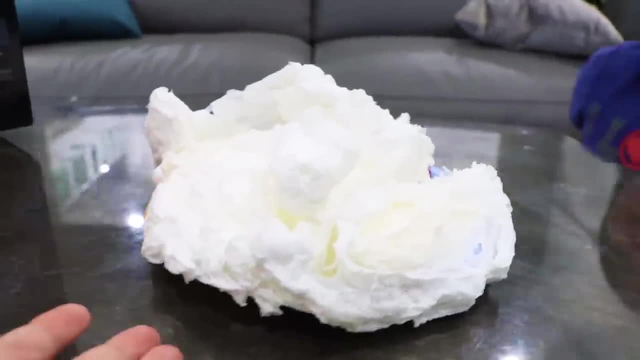 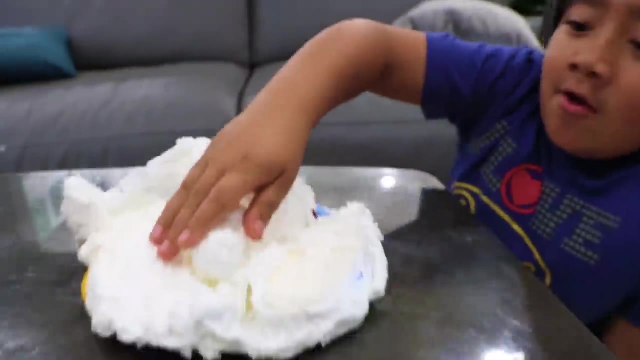 Got it. It looks like toilet paper to Ryan. It looks like a lot Kind of looks like whipped cream. Yeah, Let's see. Okay, so safe to touch. now Ryan, Touch it and see what it. Whoa, What does it look like? 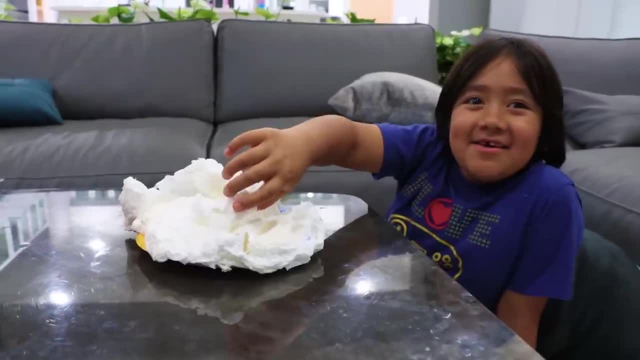 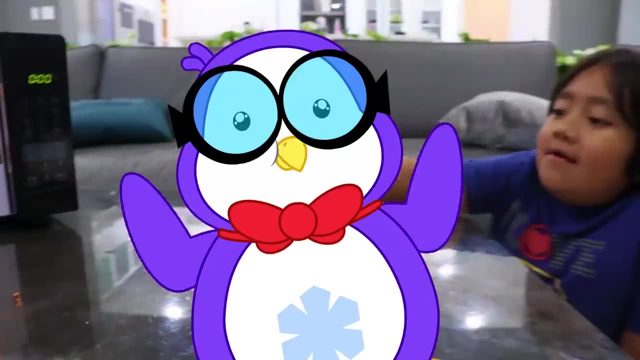 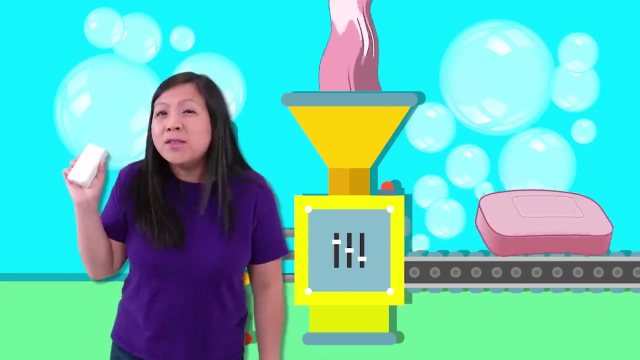 It feels like maybe cotton candy, Really. Yeah, Wow, Just a little bit more rough. Yeah, so this one actually only works with ivory soap. But wait, I don't understand. How does it work? Yeah, So why did the ivory soap expand in the microwave? When it was made. there are air that is trapped inside the mixture And because of the air, that's why it floats in water. So when you put the soap in the microwave, the air and the water molecules that was in the soap starts to heat up, vibrate and expand. 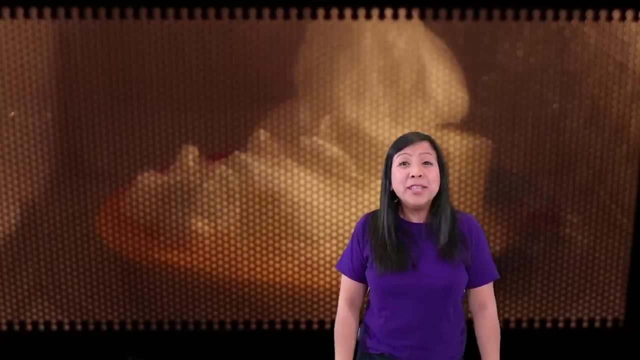 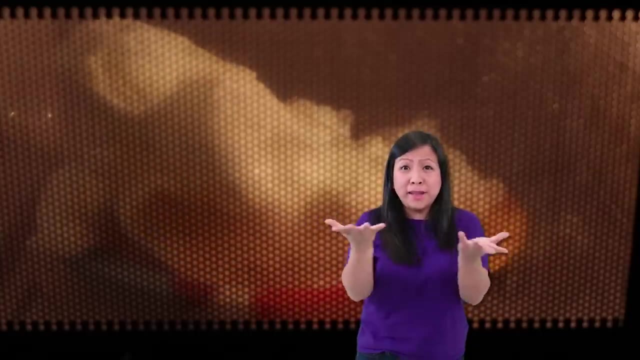 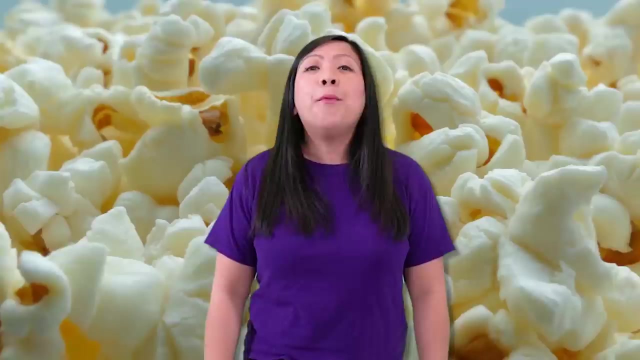 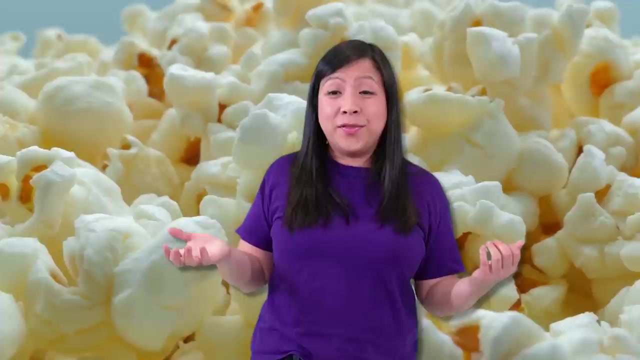 and spread farther apart. They pushes against the rest of the soap molecules, expanding the bar into a fluffy cloud blob. Do you guys like popcorn? It works the same way. Water inside the kernel expands and pushes on the walls as it's being heated inside the microwave. 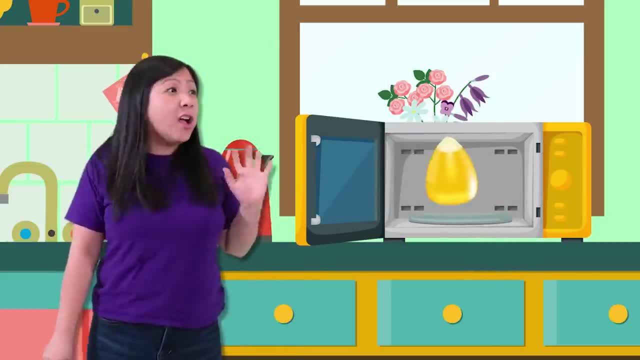 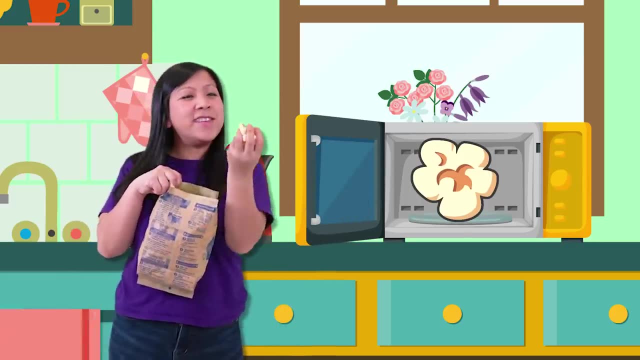 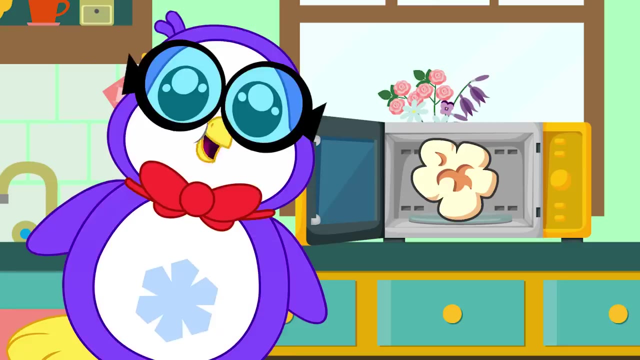 The water will turn into steam and expand and pushes along the wall of the kernel until, pop, The kernel explode and we have a yummy piece of popcorn. Mmm, that was so cool. Let's get back to Ryan. Now Emma wants to touch it. 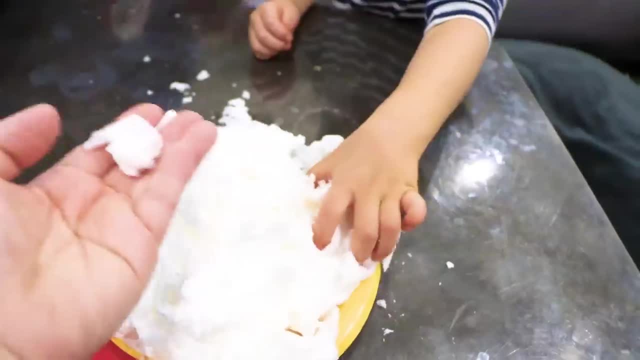 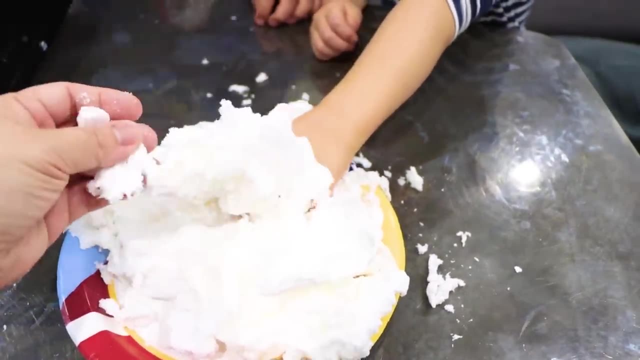 Yeah. so, Emma, this is soap. Apparently, It's like coming apart. Why do you microwave it? Well, because I wanted to show Ryan how soap expands when you microwave it. Look see, But it's all mushy. I ruined my fingers.